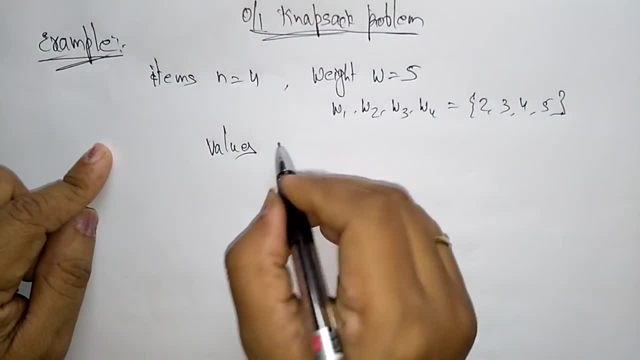 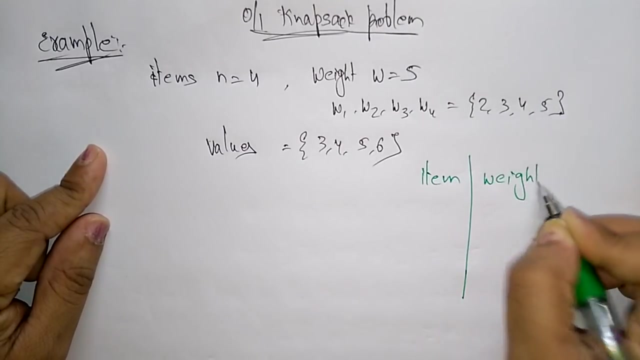 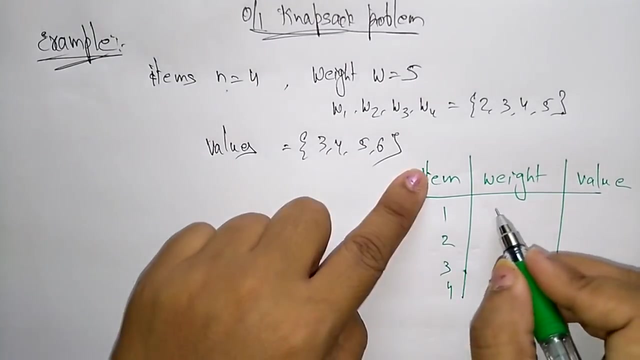 And those values. let us take values, or for those particular weights, is 3,, 4,, 5, 6.. Even this can also represent the weight. This can also be represented like tabular form, Like item weight and the value. So total, how many items? 4 items 1,, 2,, 3,, 4.. And the respective weights are 2,, 3,, 4, 5.. 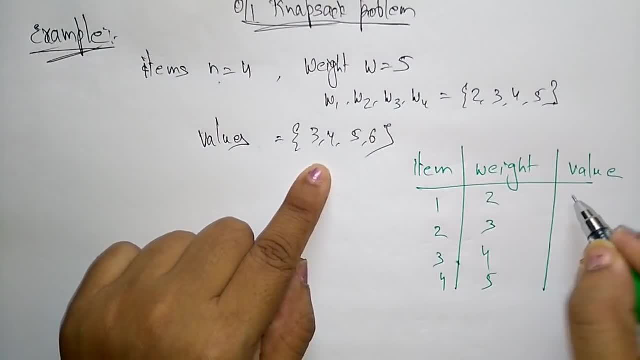 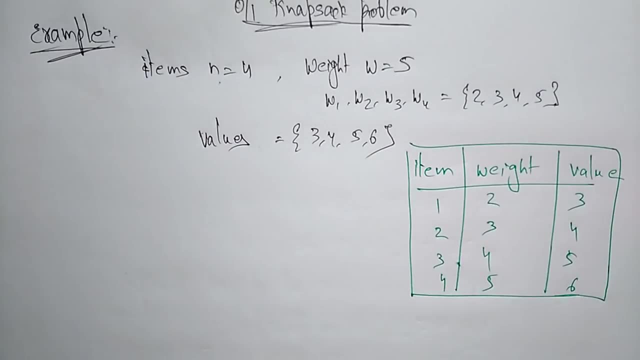 And the values for those weighted items are 3,, 4,, 5,, 6.. So this can also be represented in tabular form. Now let us calculate The weights means we have to be get the optimal solution that has the less maximum weight that knapsack can handle. 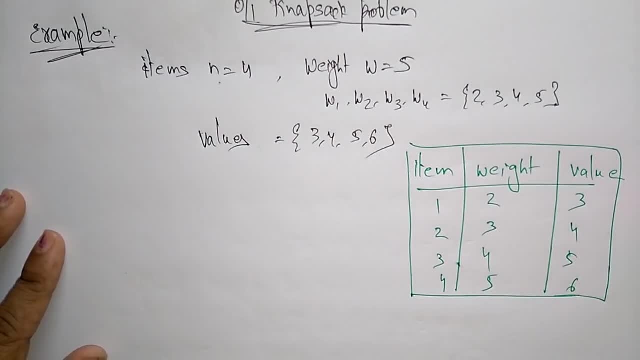 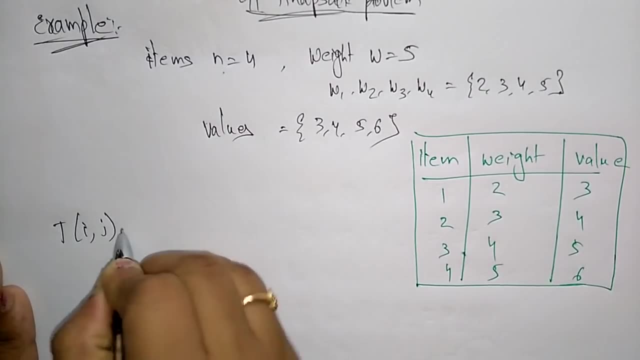 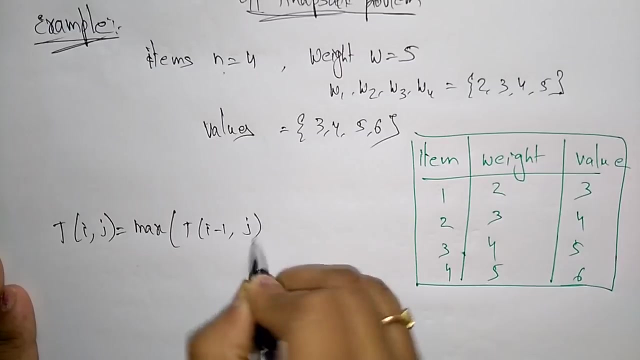 And what are the items that he can insert in the knapsack That we have to be find out. So for this the formula is The maximum value of I plus t, of I minus 1 comma, j minus weight I. So this is a formula that we are applying for finding out the knapsack problem. 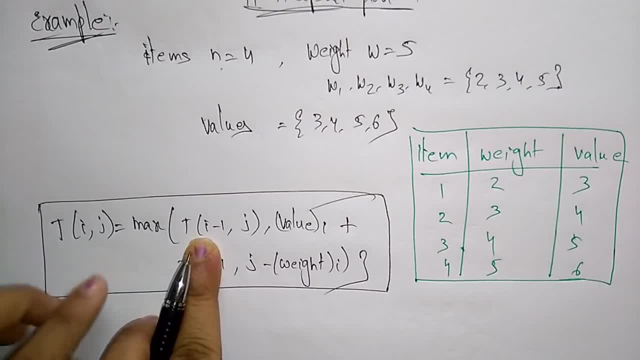 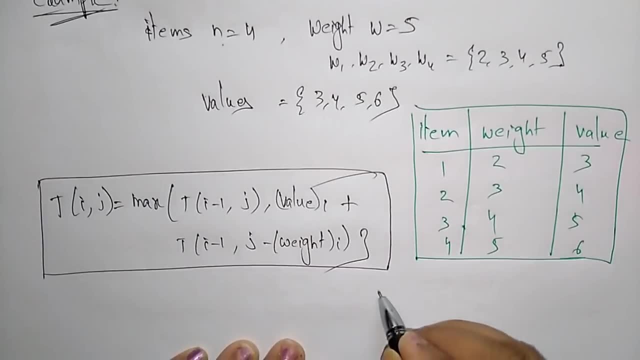 So here the t of I comma, I minus 1 is nothing but the maximum values of selected item. The maximum value of selected item. So for this we have to be considered a test. So now we are going to discuss правильно. 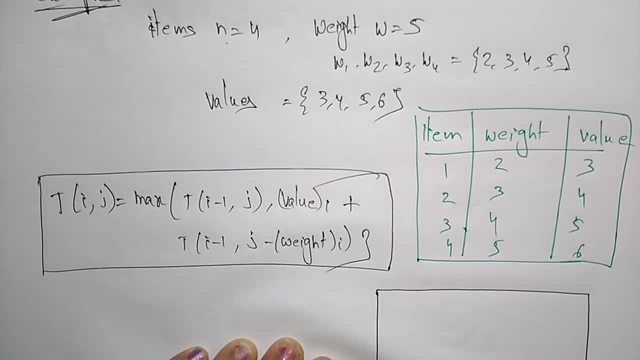 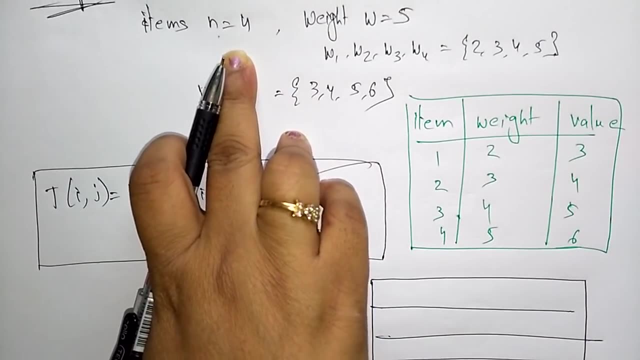 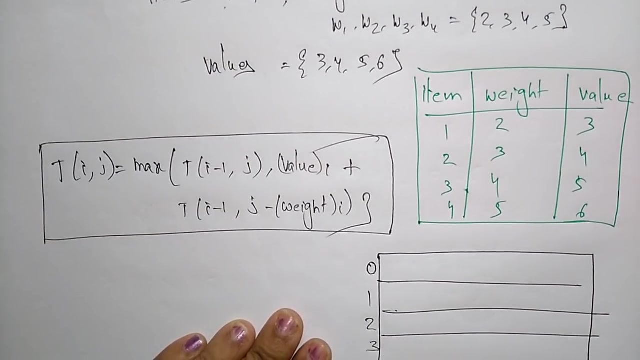 So our test: here we are going to all these, so let us take a matrix. here total, we are having the four values, so we have to take 5, 0, 1, 2, 3, 4, okay, and here that weights, here total the weights. 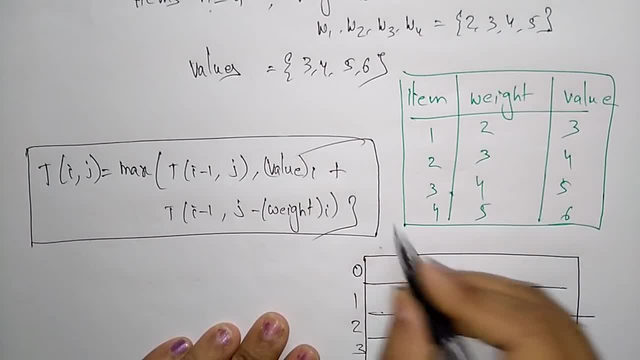 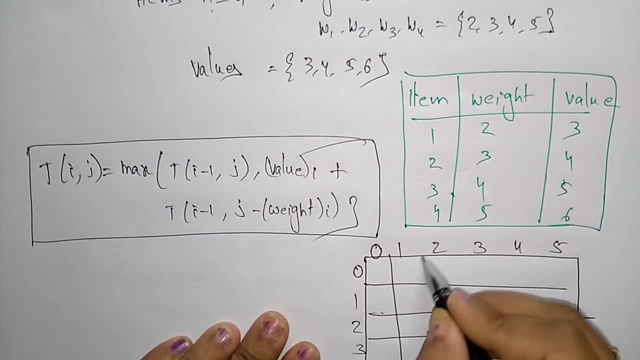 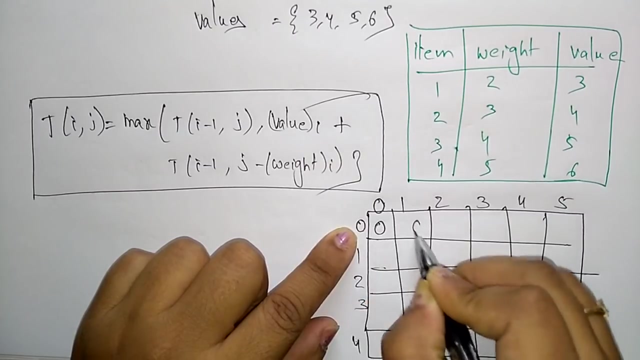 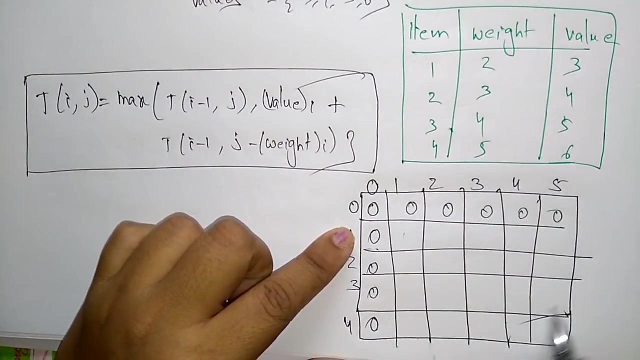 are five, four weights. so let us take five zero, one, two, three, four, five. okay, so the starting, all I value of the zero is zero, and here you may mark it as all zeros. okay, now we have to be calibrated. only this part, because the item one and 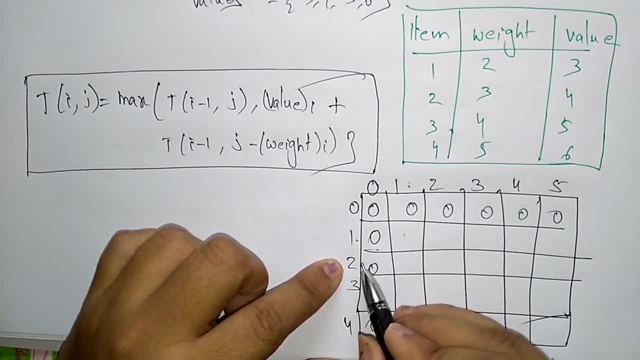 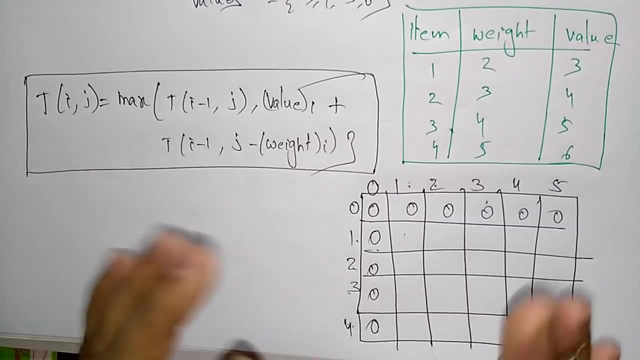 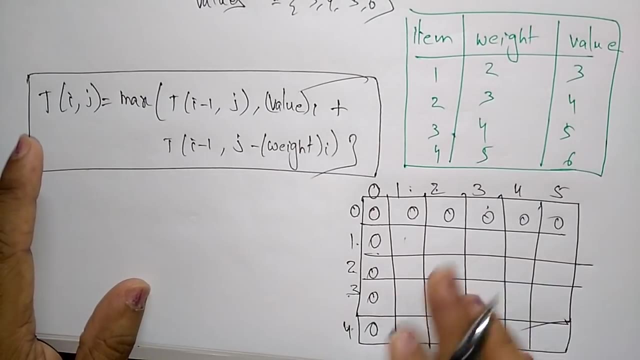 the weight: weight of that item one, item two and the weight of that item two, item three, the weight of item three, item four and the weight of item five. so, like that, we have to be calculate everything here, okay, from starting from this. so to make this as they just, we are inserting the zero here. now just apply the formula and we: 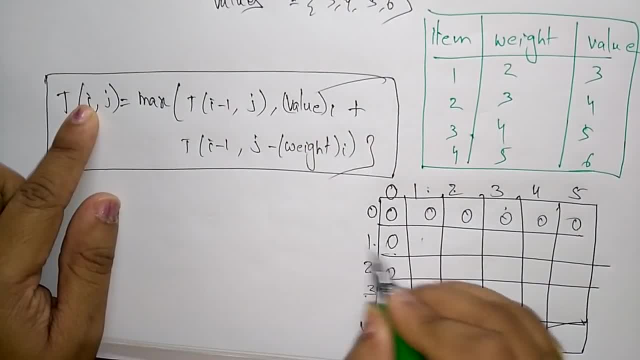 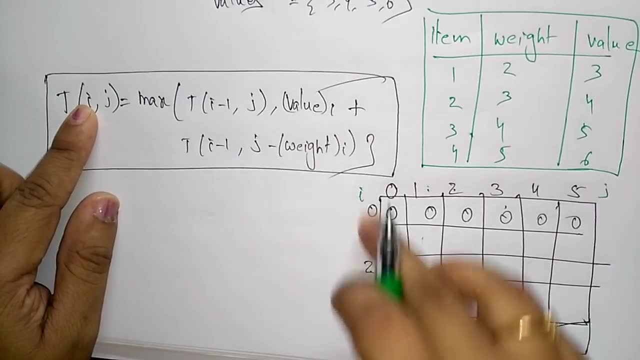 have to fill all those things. so the first T, this is I and this represents this complete row represents that, the columns represents the columns and the columns represents the columns and the columns represents J and rows represents the I. so first we have to find out this: that 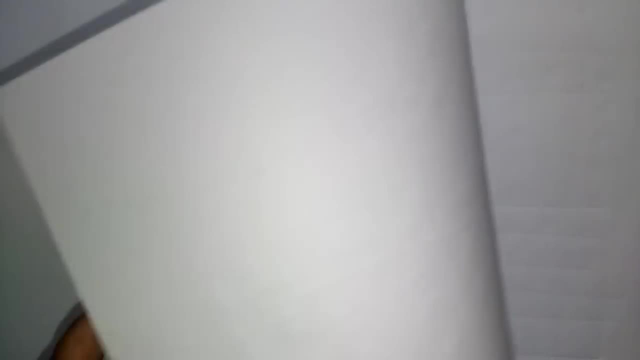 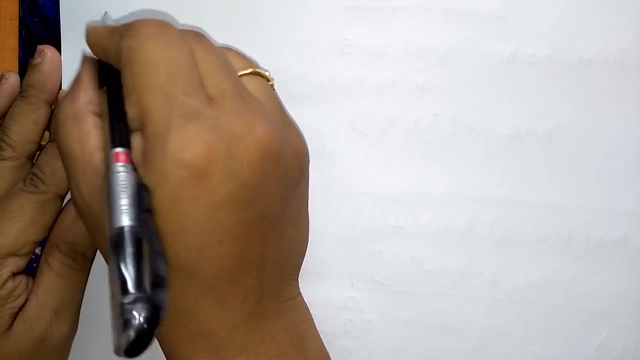 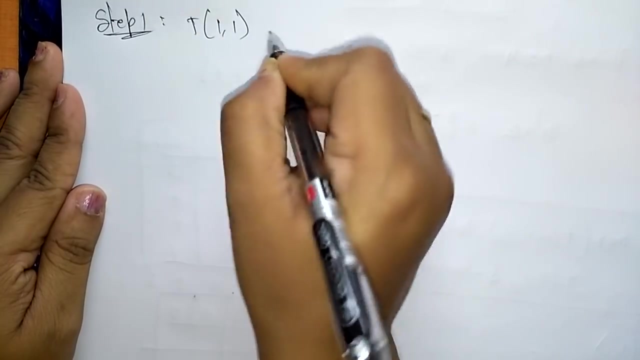 is T 1 comma 1? we have to be find out. so let us take solve the problem step by step. let us start by drawing a table. now take the step 1. we have to find out T 1 comma 1. so here, this is I and this is J. I is 1 and J is 1, so we have to find. 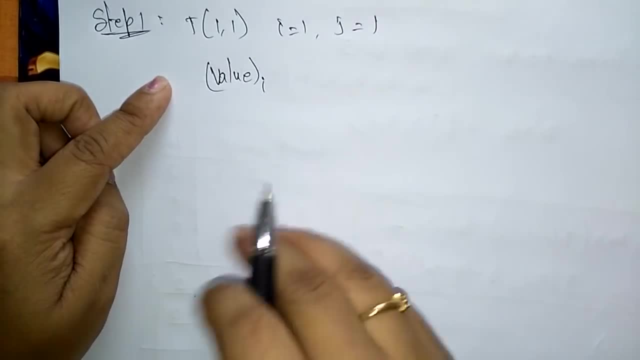 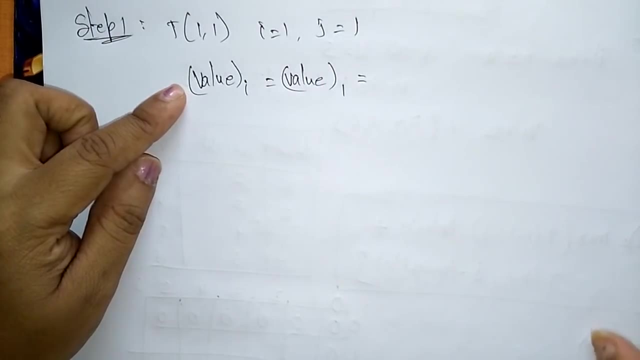 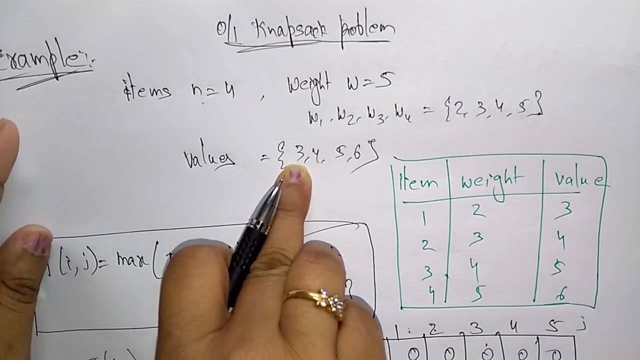 out the value of I, so that these values, these should be substitute in the formula. value of I, that is value of 1. so what is the value of 1? so that already I will write it here: the value of 1 is 3, so the value of first item is 3, just. 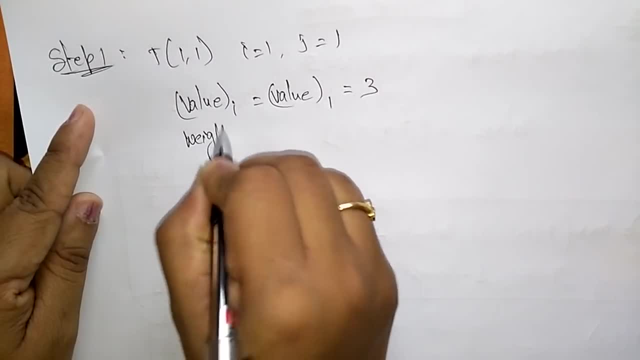 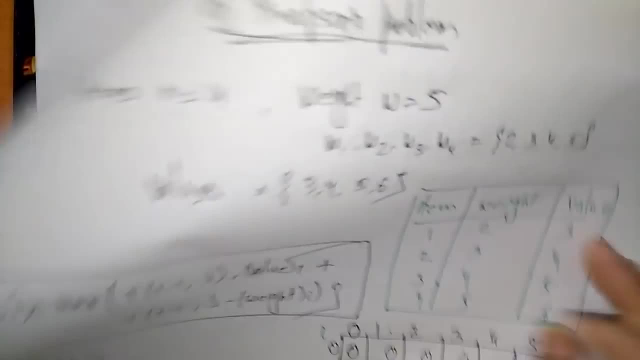 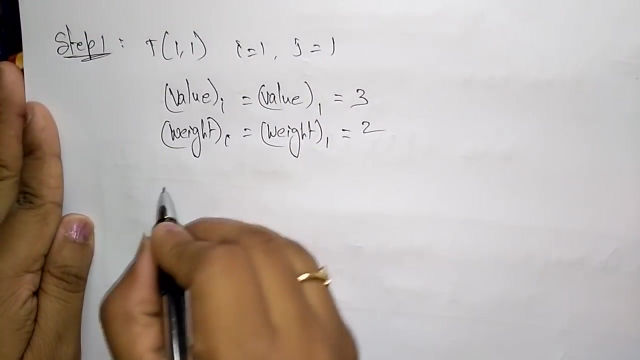 write value of this and weight of I. that is the weight of 1. what is the weight of 1? so weight of the first item is 2. so just write the 2. now substitute these values in the formula so that we get T of 1 comma. 1 is equal to maximum of T of. 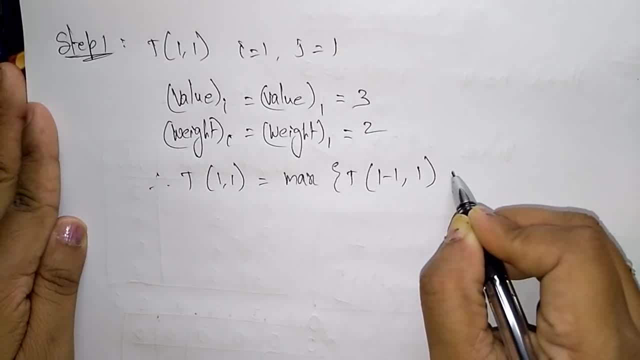 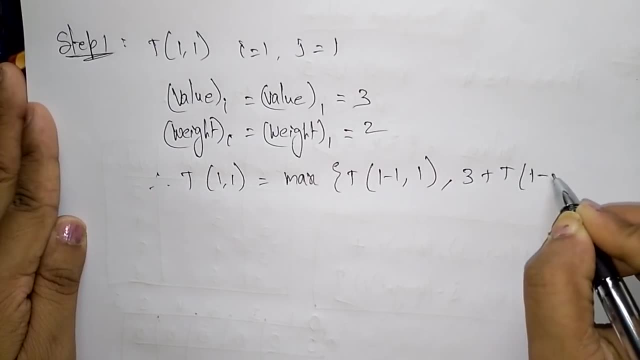 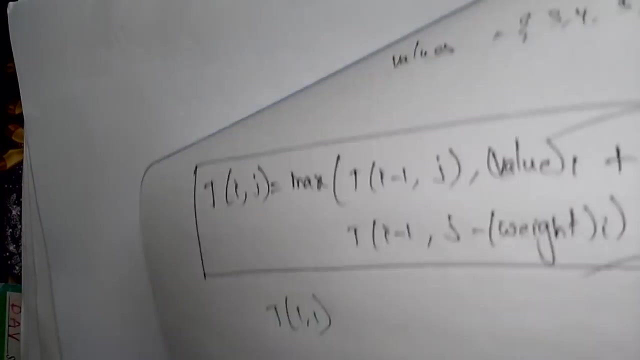 1 minus 1 comma, 1 comma 3 plus T of 2, 1 minus 1 comma, 1 minus 2. so just I substitute to the values, whatever the formula that I had given here for calculating the knapsack problem. so for 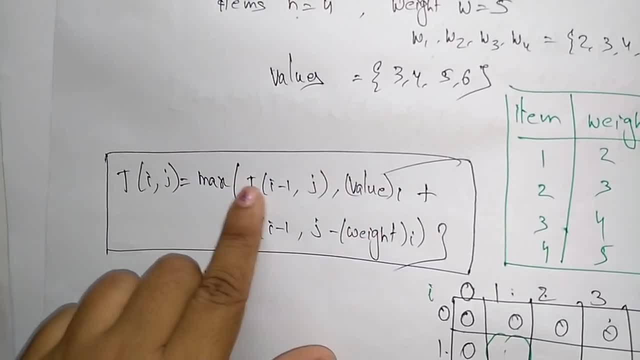 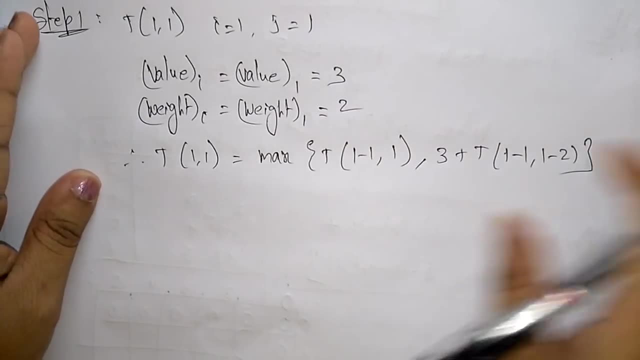 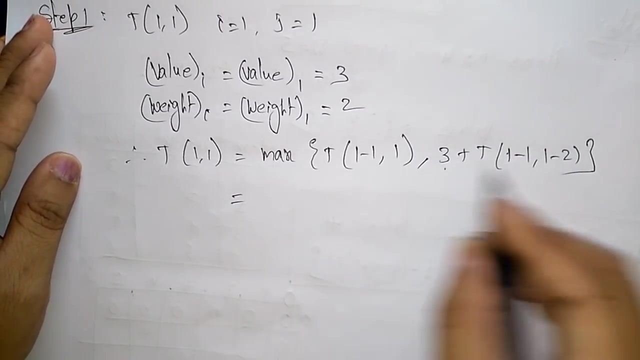 value of I and weight of I and substitute the values- and I is 1 and J is 1, just substitute the value of I 1 and J 1 here. so we'll get like this: so this is the weight, so this is the value and this is the weight we get. this is the value and this. 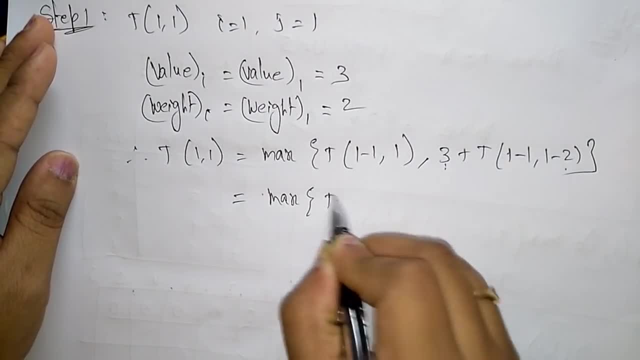 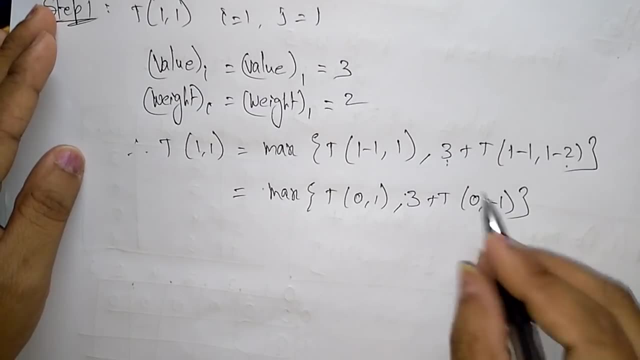 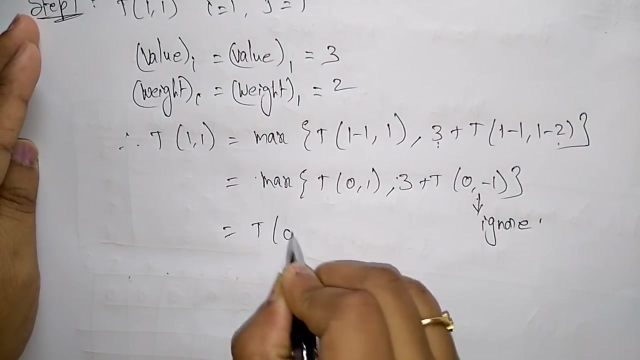 is a weight maximum of T of 0 comma 1 comma 3, plus T of 0 comma minus 1. so we get the minus 1 as a weight. so just ignore, if we get the minus 1 we won't take them negative weights. so finally, T of 0 comma 1. so what is the value of T? 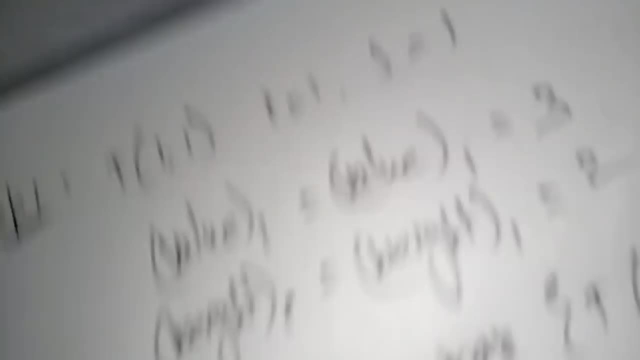 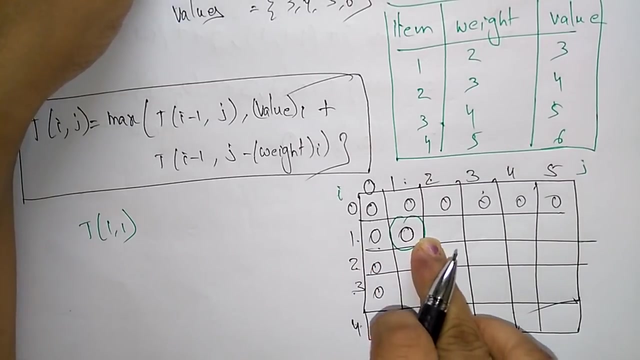 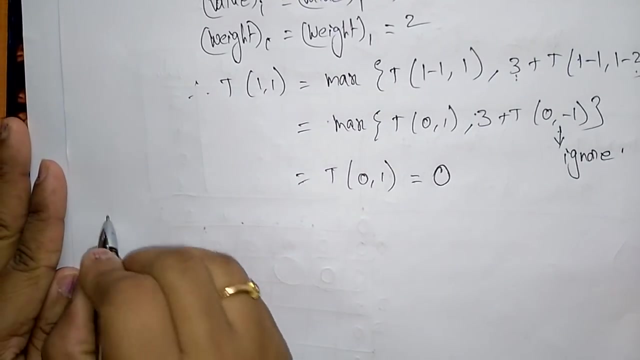 of 0 comma 1 0. 1 is 0. T 1: 1 is we get 0. now calculate T 1- 2. next we will calculate row wise. so next is T 1, 2. so step 2. so apply the same formula: T 1, 2. i is equal to 1, j is equal. 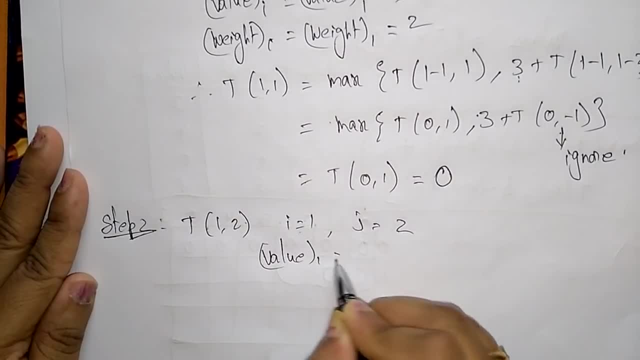 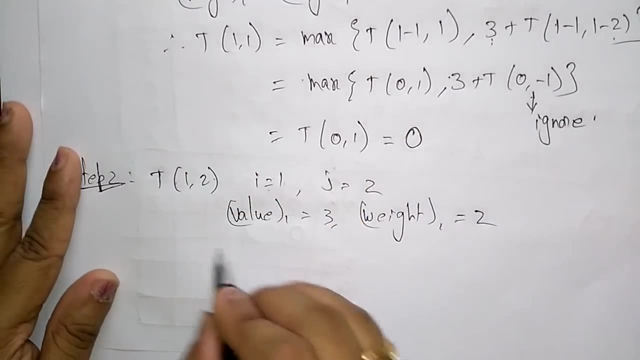 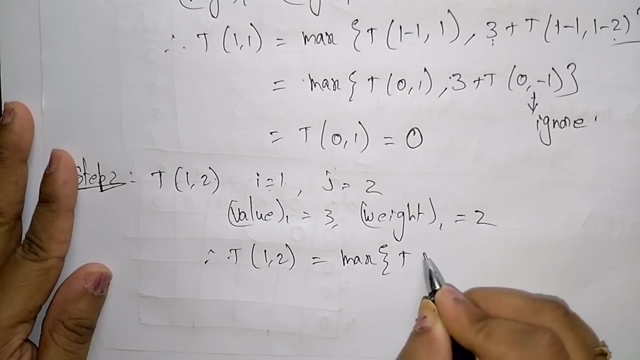 to 2. so value of i, that is a 1, is 3- we know that- and the weight of 1, that is 2. just substitute those values till here and then I will be able to write this into this. in the equation, t of 1 comma 2 is equal to maximum of t of, we get the 0 comma 2 comma 3 plus t of 0. 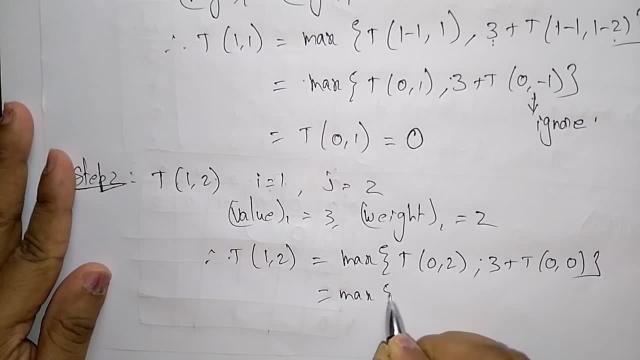 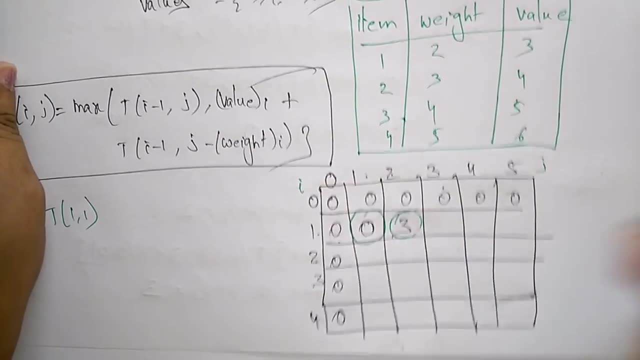 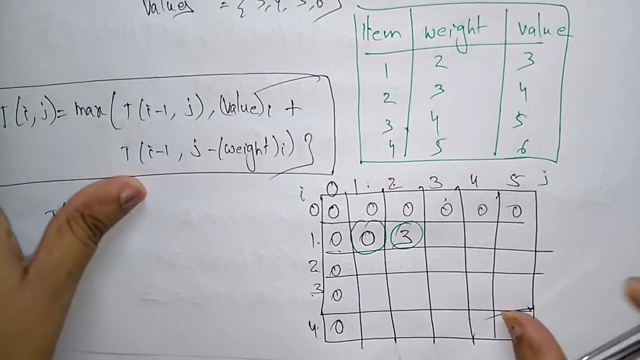 comma 0, then maximum of 0 comma 3 plus 0, so maximum value is 3.. So just substitute the 3 value here. So in the same way we have to be calculate 1 comma 3.. So just calculate the step. 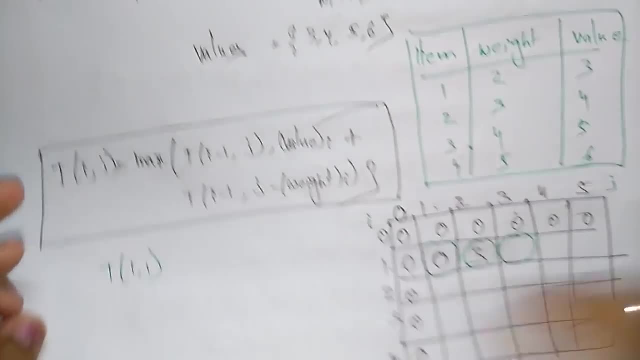 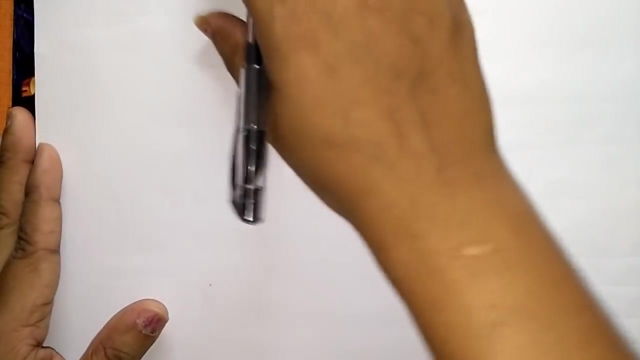 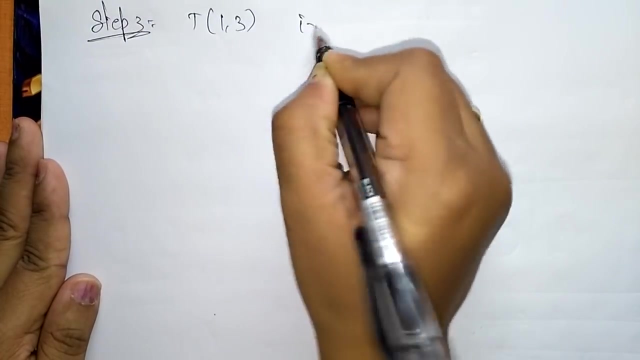 3, that is a, we have to calculate 1- 3.. So like this: first we complete first row, second row, third row, fourth row, like that. So next is 1 comma 3, step 3: t of 1 comma 3. so i is equal to 1, j is: 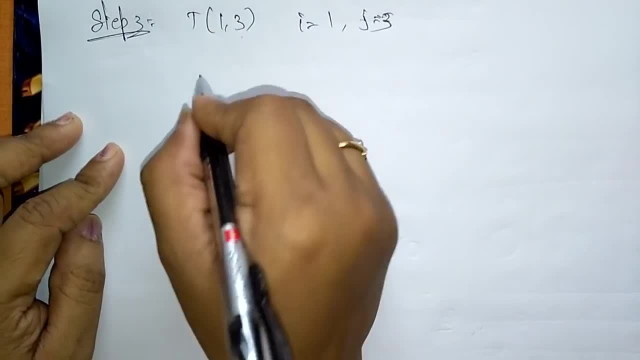 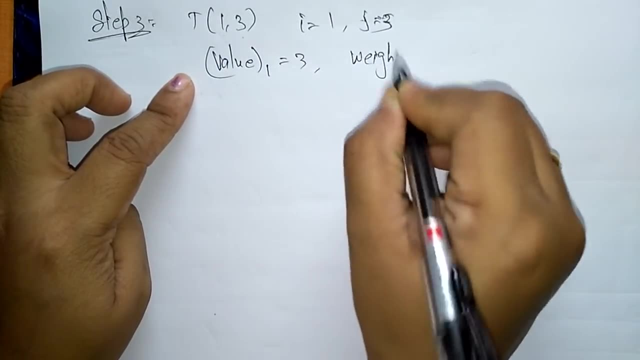 equal to 3, i, 1, j, 3.. So value of 1: we know that value of i, that is a value of 1, is 3 and weight of i, That is the weight of 1, is 2.. Therefore t of 1 comma 3 is equal. to substitute those values we. 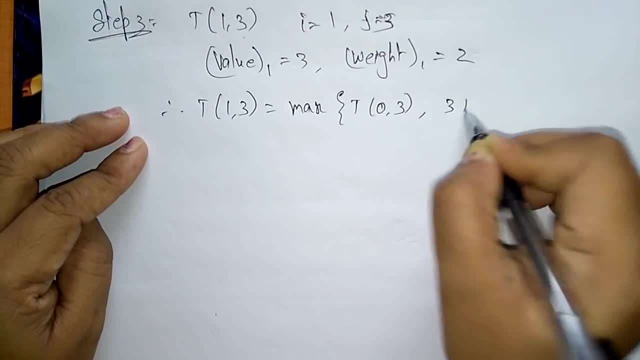 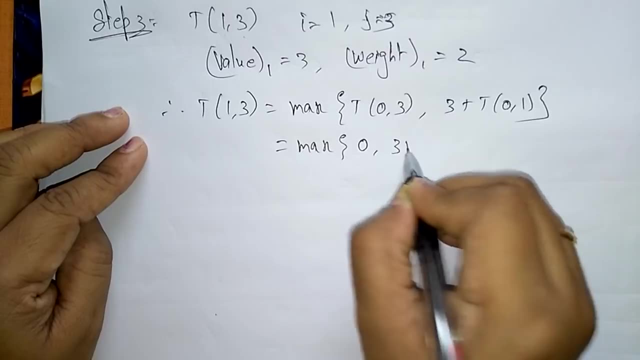 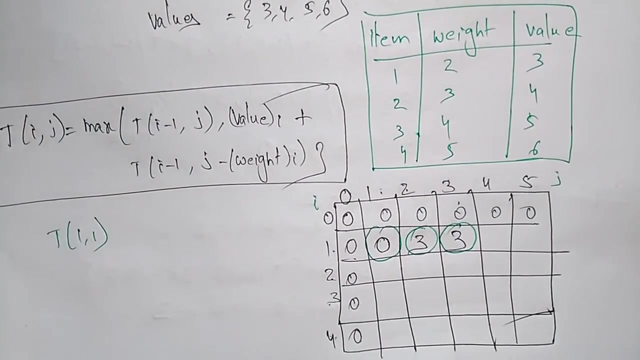 will get t of 0 comma 3 comma 3 plus t of 0 comma 1.. So for those values, 0 comma 3 is 0 and this is 3 plus 0. So maximum value we will get t of 1- 3 is 3.. Just write 3 value. So next t 1- 4.. 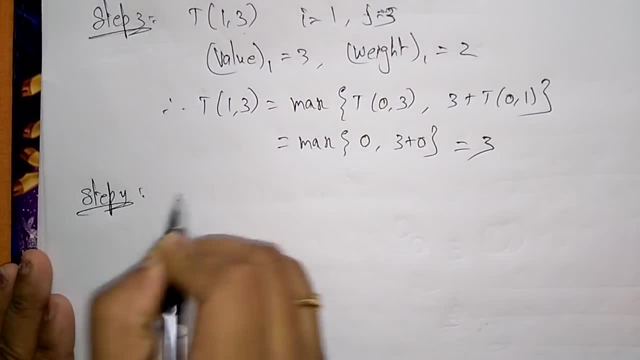 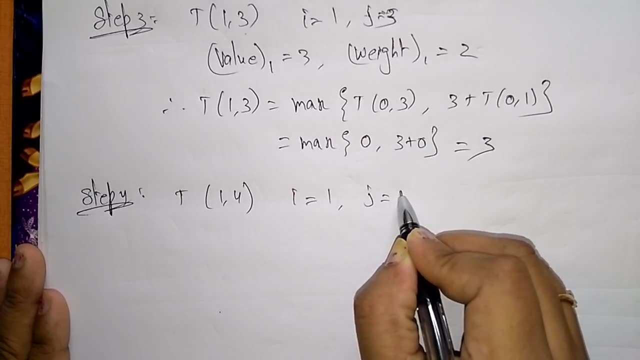 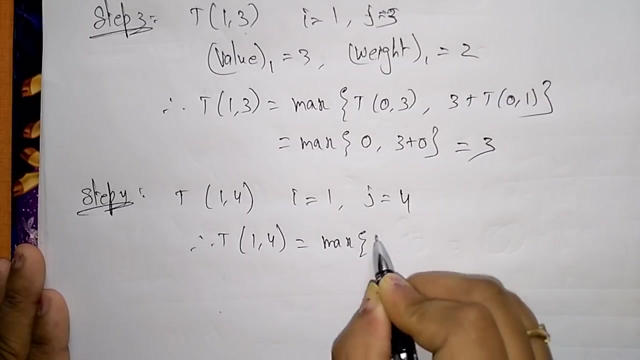 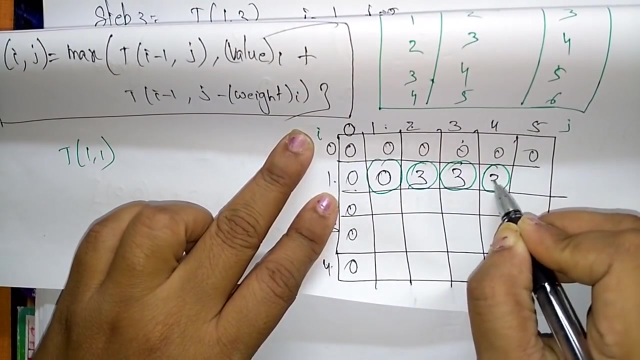 This is step 4.. t of 1 comma 4, i is equal to 1, j is equal to 4.. Substitute those values, t 1 comma 4, we will get the maximum of just. I am writing directly: 0 plus 3, 0, we will get 3.. So for this we get again 3.. 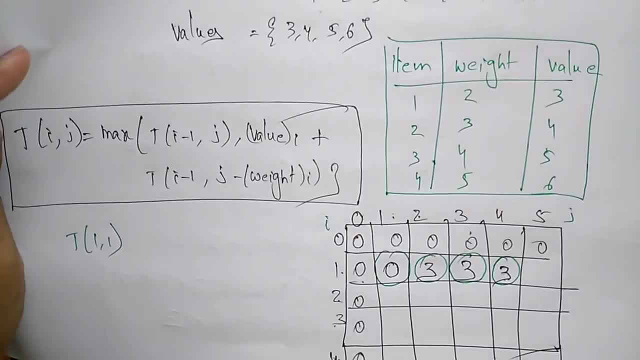 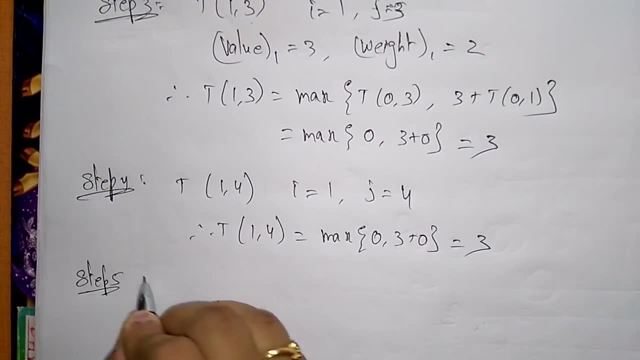 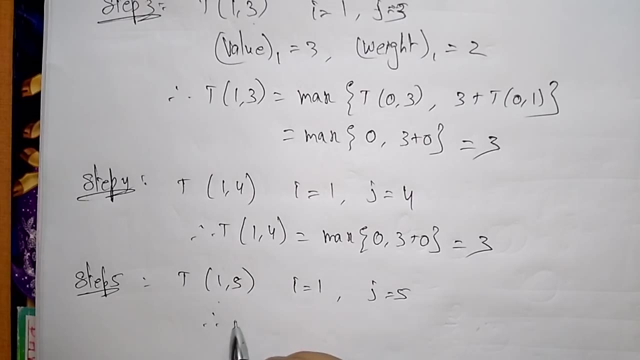 And next, next value is t, 1 comma 5.. Now calculate the step, Step: 5: t of 1 comma. 5. i is equal to 1, j is equal to 5.. And value of the same values we will get: i is 3 and weight. j value is 3 and weight is 2.. 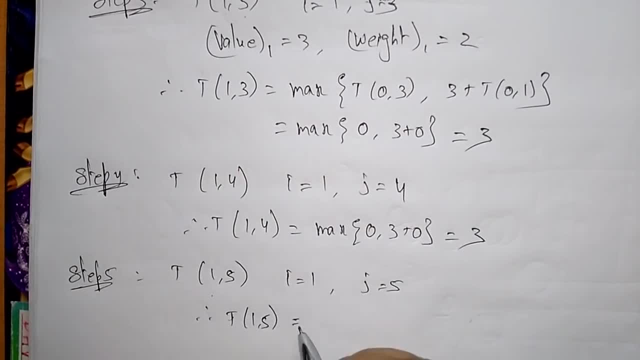 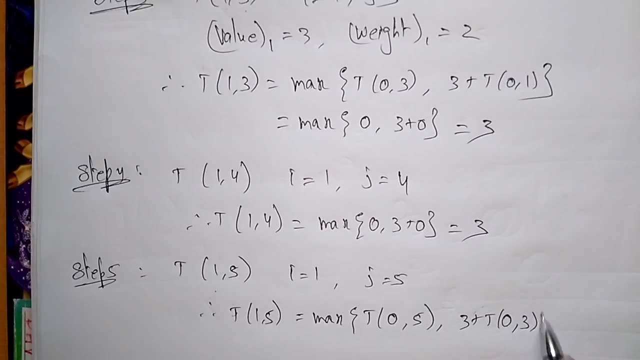 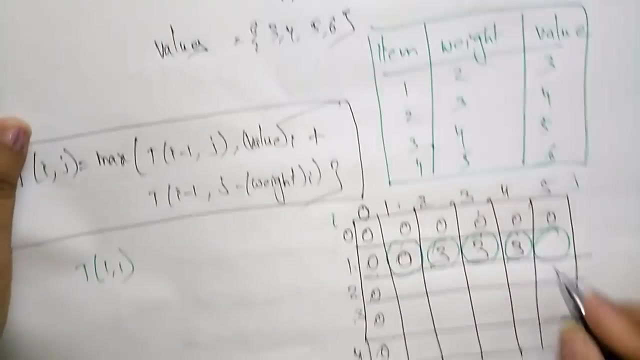 For the first item, t of 1 comma 5 is equal to maximum of t of 0 comma 5 comma 3 plus t of 0 comma 3.. That is the maximum of 0 comma, And again we will get 3 plus 0.. My value is 3.. So this row is over. Now coming to this row, The second row. 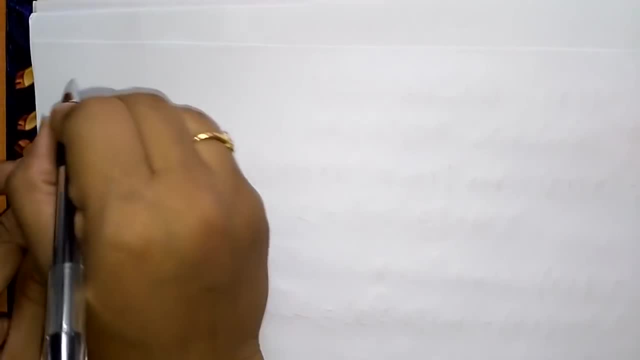 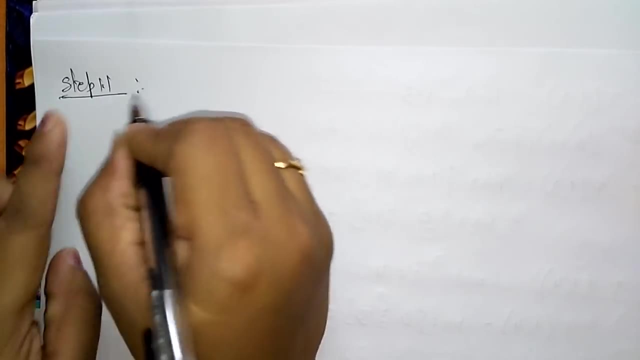 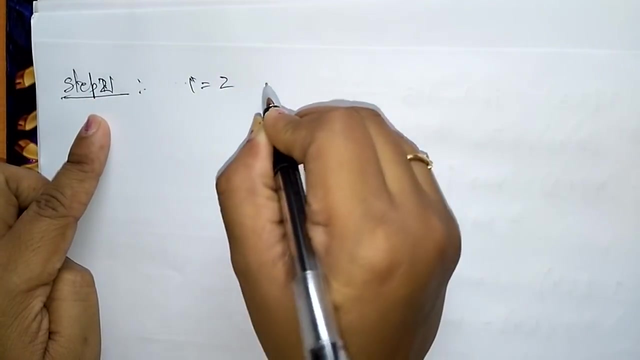 So in the second row we have to be take, let us take step 1, point 1: 1.. So previously I take 1, now we take second, The second row. Next take 2: 1.. The second row So we have here, i is equal to 2 and j is equal to 1, because the second row is. 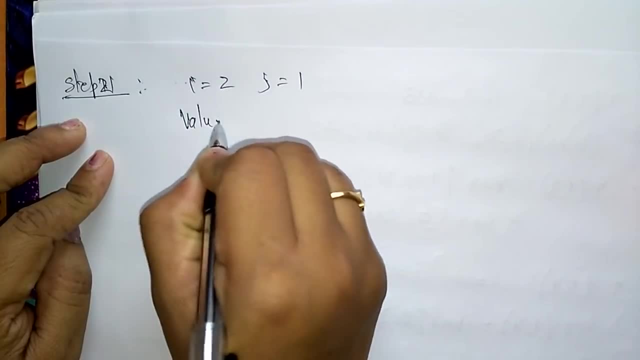 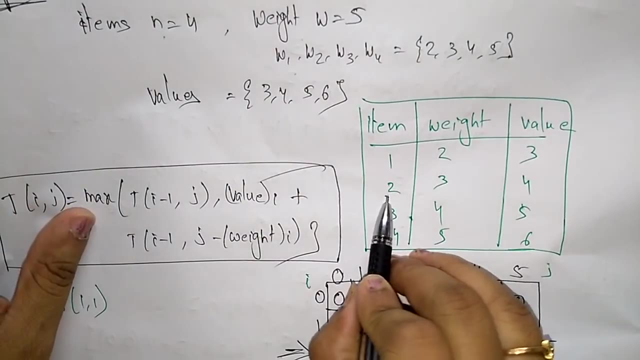 2 and the column is 1.. So for this value of i, that is, the value of 2, is 4.. So, how we know, the value of 2 is 4.. So this is the item. Item of 2 is, value is 4 and weight is 3.. 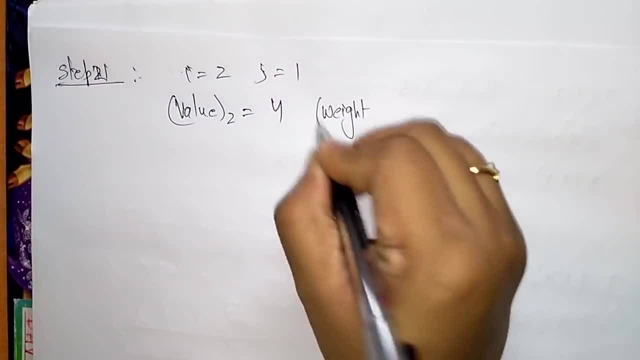 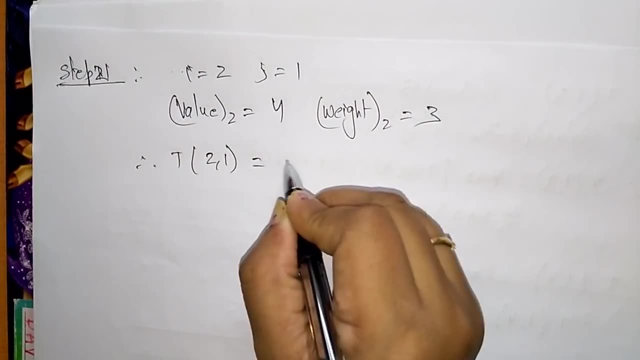 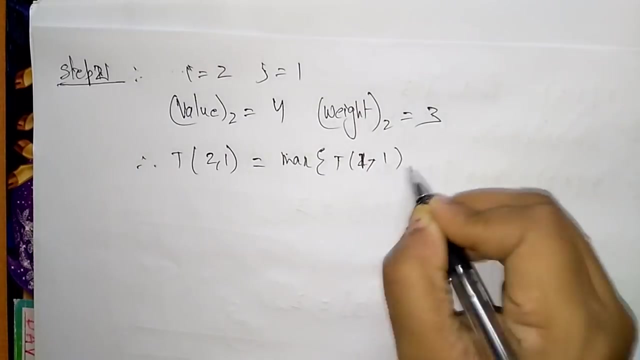 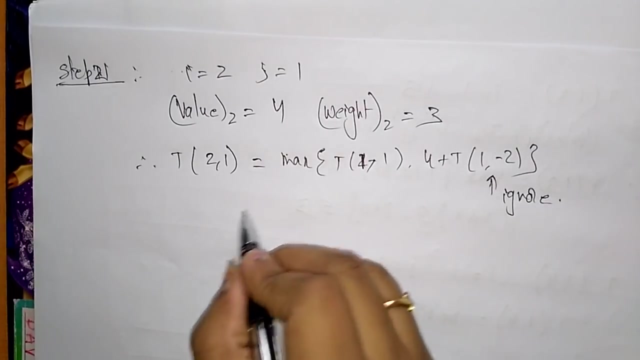 So now just write that Weight of 2 is 3.. So just substitute t of 2 comma 1. we will get maximum of t of 2 minus 1 comma 1.. Basically I am writing 1 comma 1 comma 4 plus t of 1 minus 2.. So just ignore this value because it is a negative. weights are not accepted by the person. 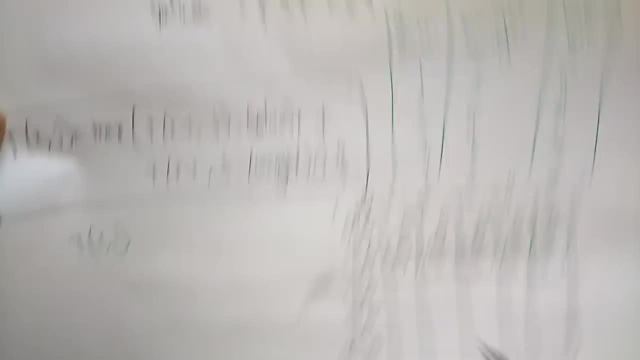 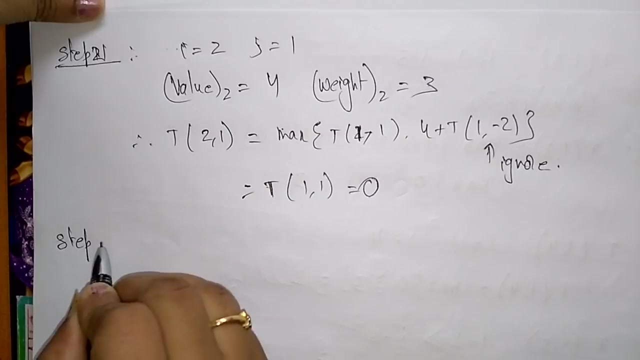 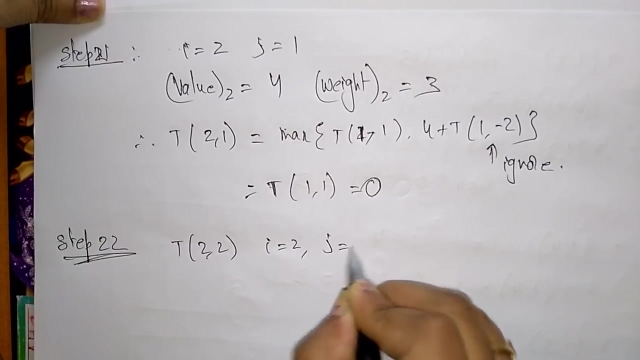 So finally, t of 1 comma 1, we will get 0. So just substitute 0 here And the next value is step 2, 2.. So we have to find out the t of 2 comma 2, and this is: i is equal to 2 and j is equal to 1.. 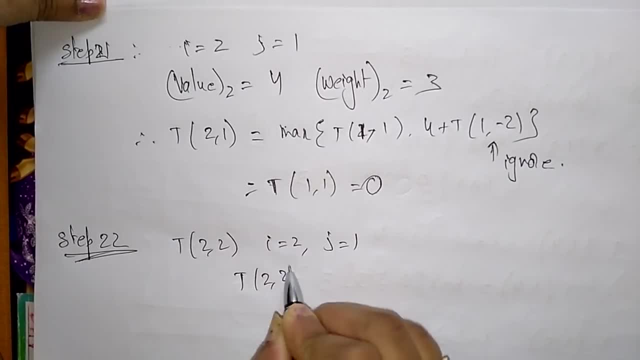 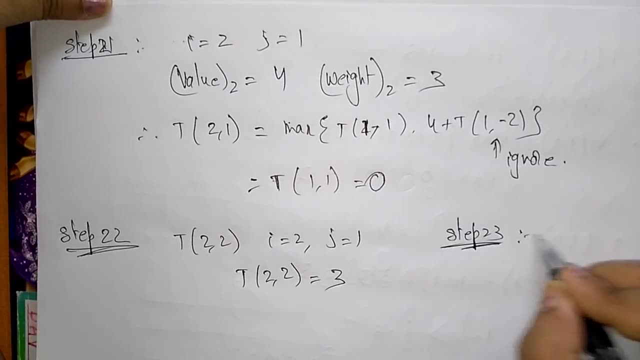 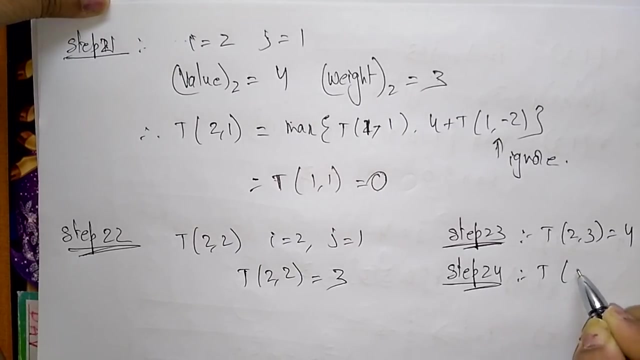 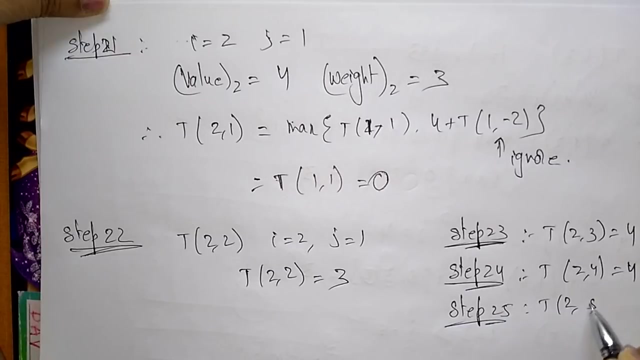 And we will get the answer As I am directly writing. we get 3 and step 2: 3. the second row and the third column will get 2 of 2, comma 3 is equal to 4 and step 2: 4, second row and the fourth column. we get 2: 4 as 4 and step 2: 5 will get 2: 5 as 7.. 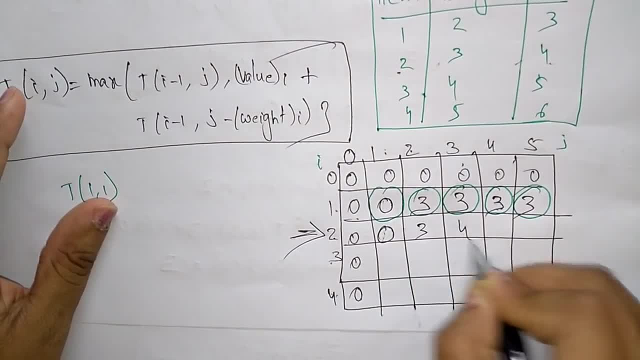 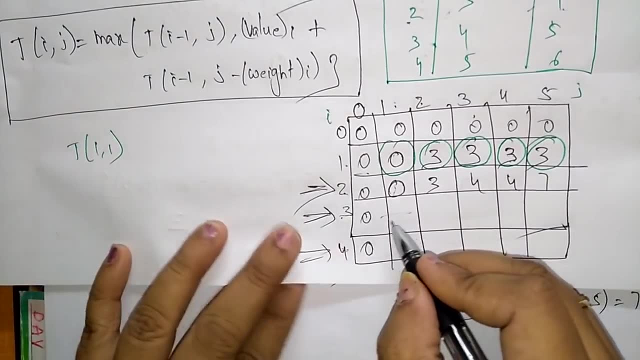 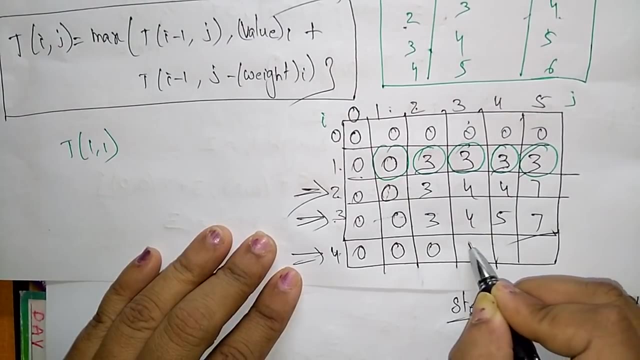 So just substitute those values: 0, 3, 4, 4, 7.. So like that, if you calculate, Next you take this row and next you take this row. the values that we will get here are 0, 3, 4, 5, 7, 0, 0. sorry, 0, 0, this 3, 4, 5, 7.. 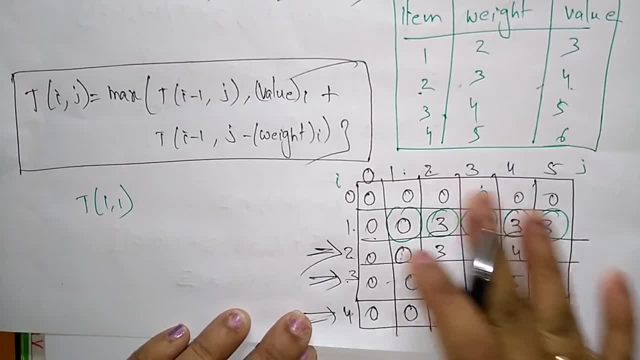 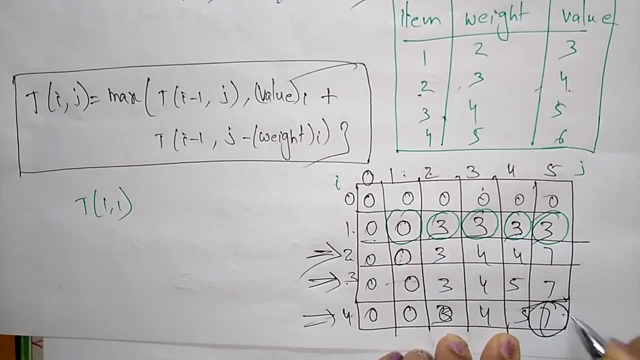 So these are the values we will get by calculating, by substituting the formula in this procedure. So here the last entry. this entry- this is- represents this: 7.. This 7 represents The maximum possible value which can he put in knapsack, means the maximum weight that he can put in the knapsack in the bag is 7.. 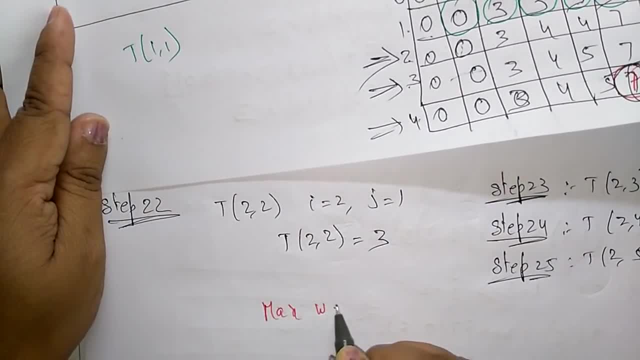 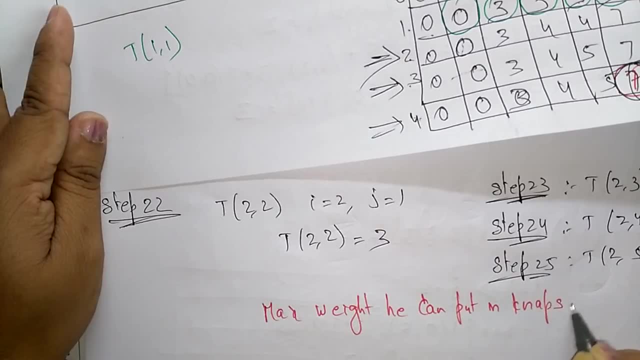 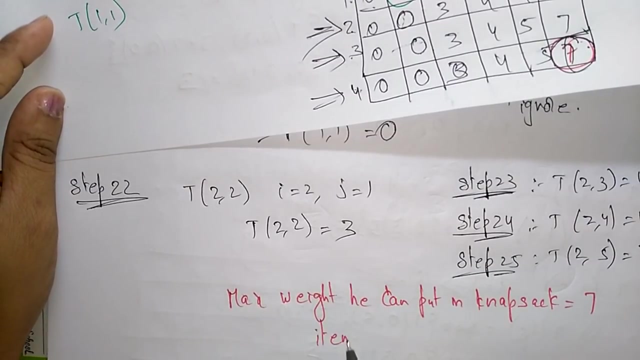 So the maximum weight he can put in knapsack is 7.. So we know that 7.. So then, what are the items that he can put in the bag items, So that we have To be find out. So the okay, the total weight he can put, the maximum weight, is 7 he can put. 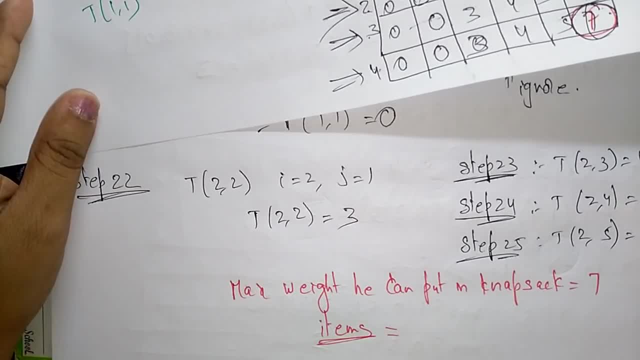 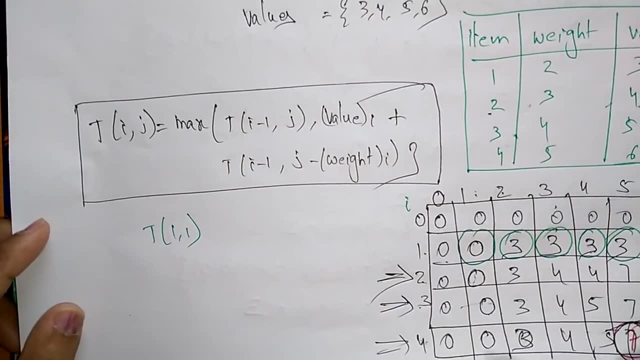 So in the total 5 values, the 5 items he can put, the maximum weight in the bag is 7- and which items he can be put. So finding the items to be in the knapsack to get the maximum possible value 7.. 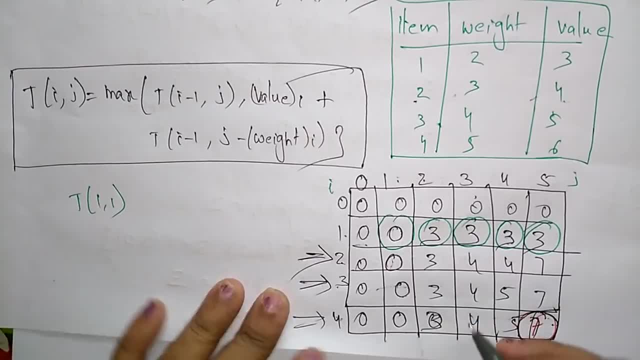 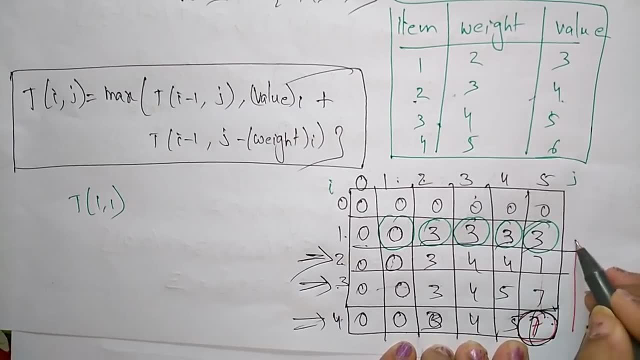 So let us consider the columns. So these are the columns. So let us consider the columns in the table. start scanning entries from bottom to up. Let us Scanning the elements from bottom to up. Okay, So while scanning, check the values with the entry. 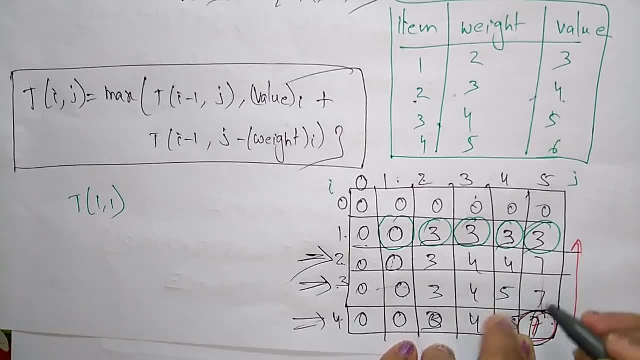 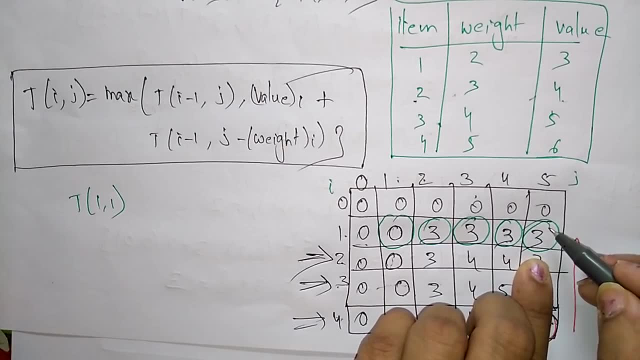 So this is an entry. check the values with the entry. immediately avoid. So this 7 is checked with this and this is checked with this and this is checked with this. So, like that, you have to be scan. So if the both the entries are same, just leave it. 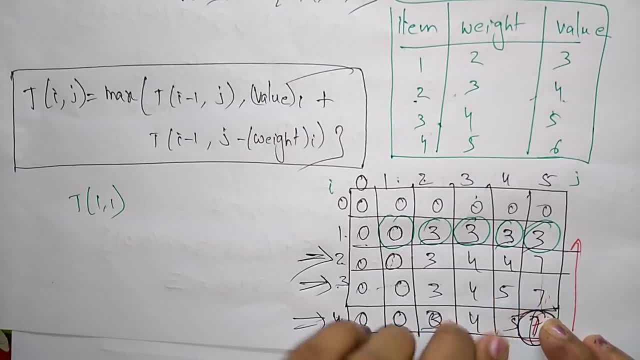 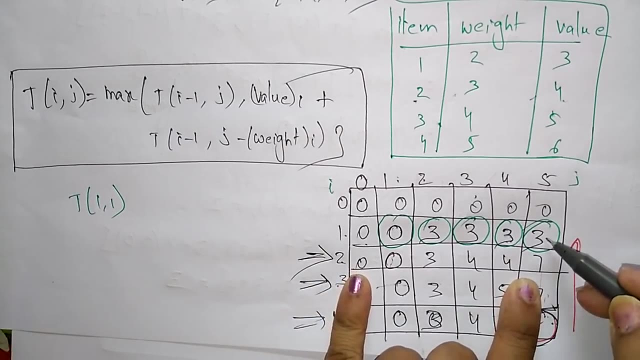 Suppose, if these entries are not matching, Okay, Then you have to mark that item, means you can select that item. So now check. So this Will be scanned with this. So both are the 7.. So don't mark this item, this item, and check this with. so the both are same. don't mark this item and check this with the 7 and 3: both are different. 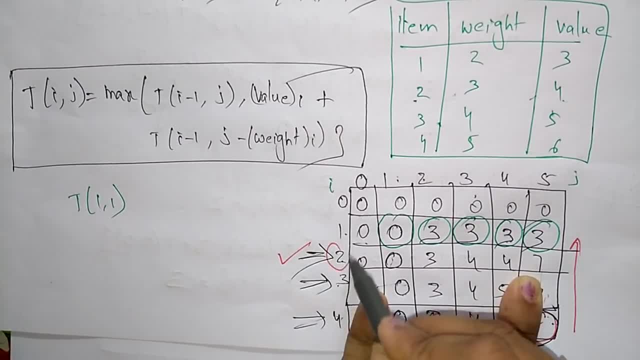 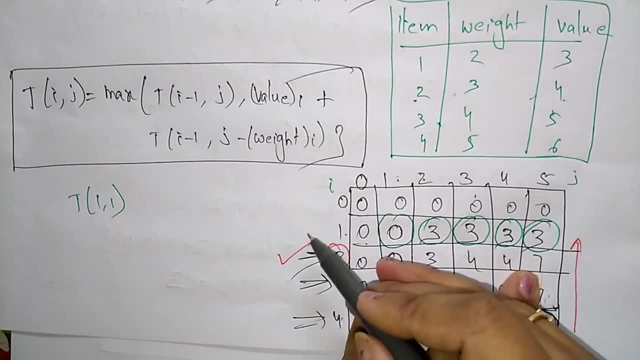 So just mark this item means the item 2 will be selected and again check this item with the above item. So here we get the 3 and this is 0. both are the different. So mark this item. So above this, there are no items, are there? 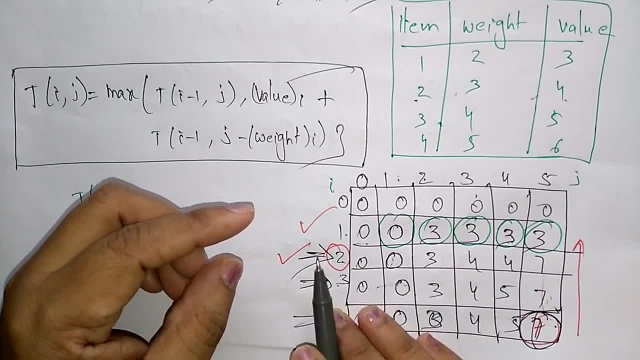 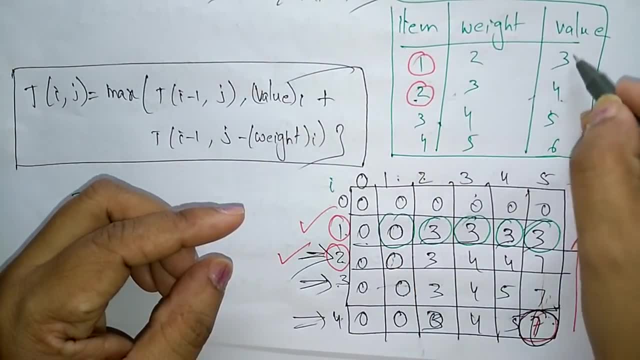 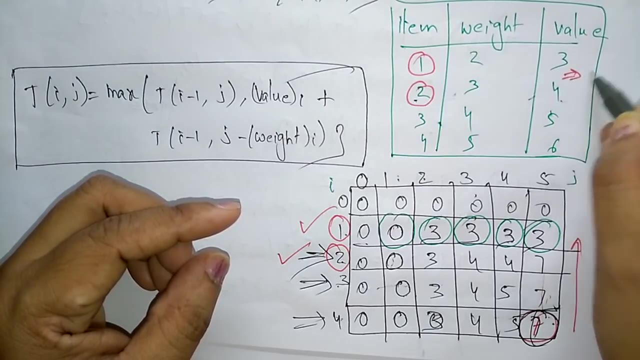 So just leave it. So the total items that he can put in The bag, or the item 1 and item 2.. So the item 1 and item 2, the total cost here for the these two values. this is a 3 plus 4. you'll get the 7.. 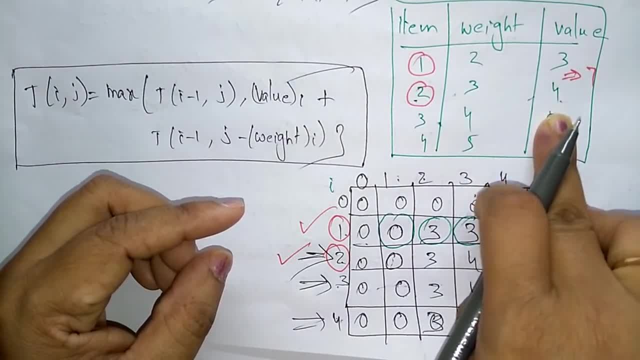 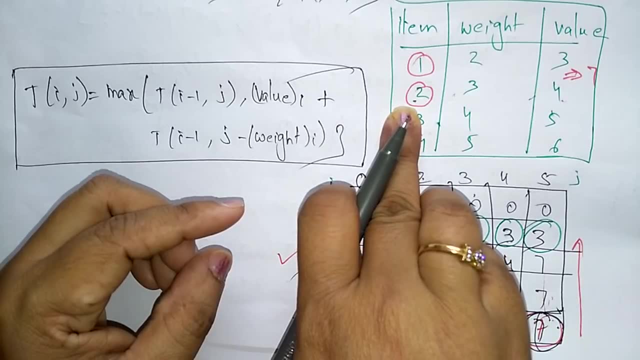 Okay, So the total maximum value he'll get is a 7 and the weights items that he can select is 1 and 2.. Okay, So the maximum weight in the bag is 5.. So the maximum weight in the bag is 5.. 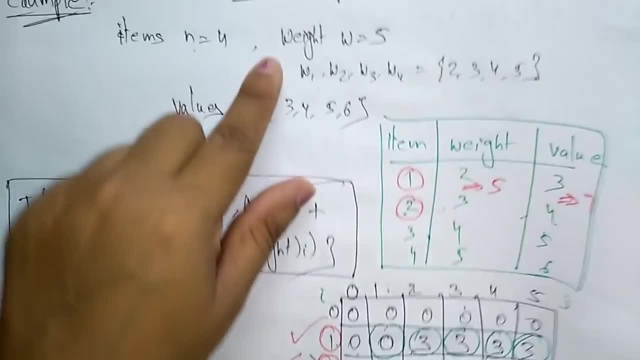 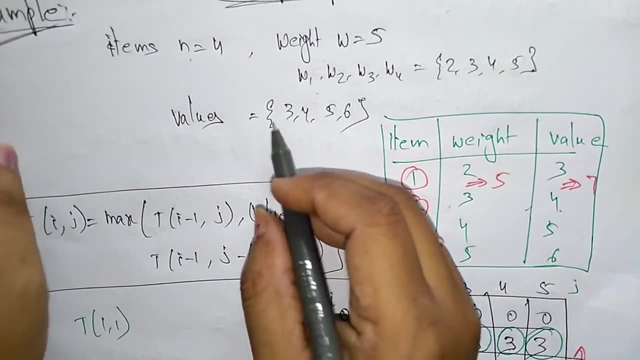 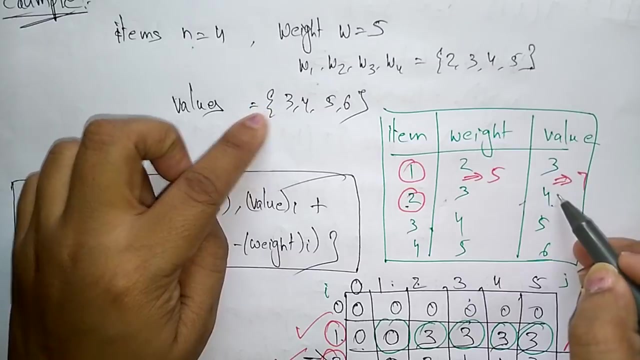 So the maximum weight in the bag is 5.. Okay, This is already given the maximum weight of the knapsack. The maximum weight of the knapsack is 5 and the values that the items that he select is the 1 and 2 items. he has to be selected and the weights for that values items are the 3 and 4..